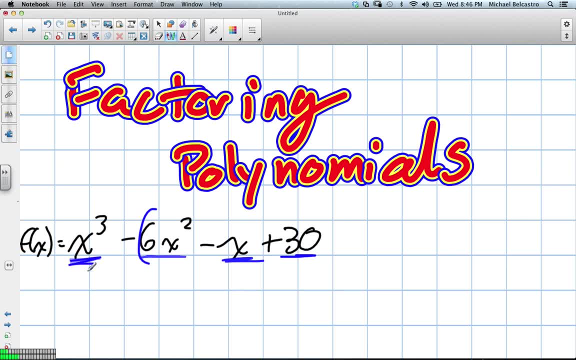 many ways of factoring stuff, but because this is cubic and we're going to have to use either synthetic or long division to solve this, we have to actually guesstimate what factors might be. What we do in order to do this is we actually take the constant term. 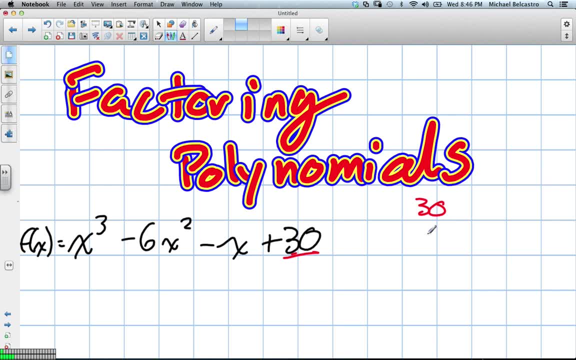 30, and we take all factors of 30.. Well, factors of 30 happen to be 30 and 1, 2 and 15, 3 and 10,. 4 doesn't go in, but 5 goes into 6, okay, So possible values we can use are plus or 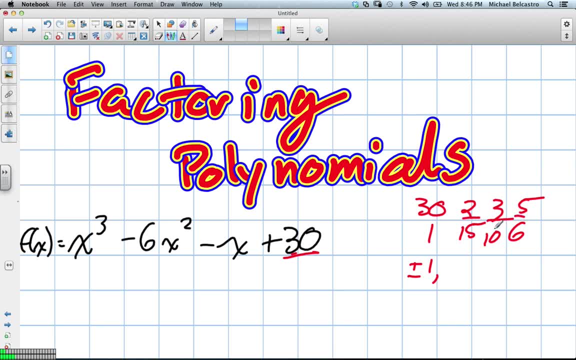 minus 1, plus or minus 2, plus or minus 3, 5,, 6,, 10,, 15, and 30. We can try all of those to see if one of them create a zero, okay. So essentially, what I'm going to do is I'm 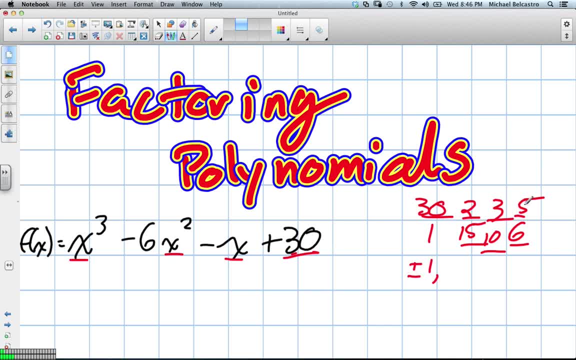 going to plug in negative 1. If neither of those work, I'm going to move to 2, plus or minus 2, plus or minus 3, plus or minus 4.. So this is a trial and error method. I'll 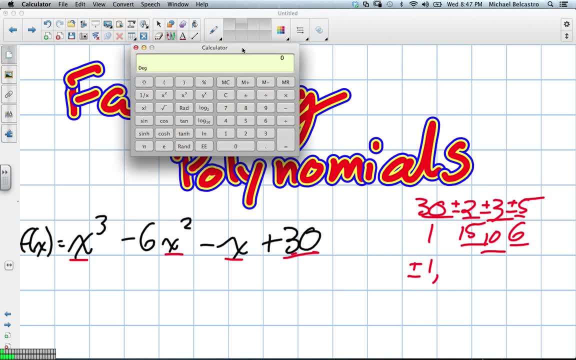 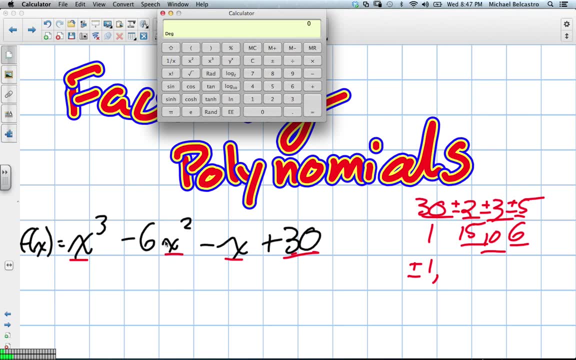 quickly go through this. Actually, I can probably tell you right off the top of my head: 1 won't work because 1 cubed is 1.. 1 squared is 1 times negative 6, so that's 1 minus 6 is negative. 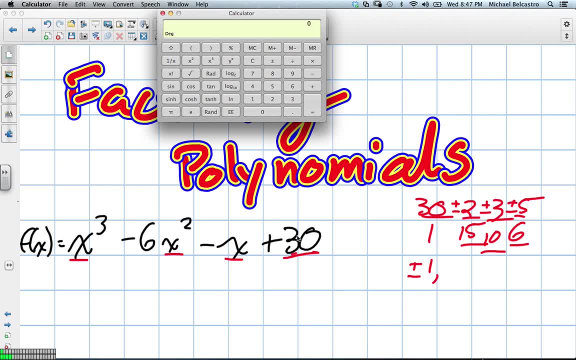 5. Minus 1 is negative. 6, plus 30 won't give us 0. So neither of the 1s are going to work, So let's try a 2. 2, maybe, Maybe, positive 2. Positive 2 cubed is 8.. 2 squared is 4 times 6 is 24.. So 8 minus. 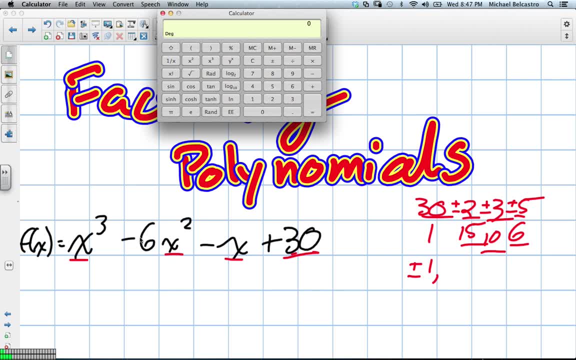 24 is 16.. Negative, 16.. Negative, 16.. Let's make sure we did that right: 2 cubed and then 4 times 6.. 4 times 6 is 24, right, Yeah, Minus 24, and then minus 2.. Minus 24, and. 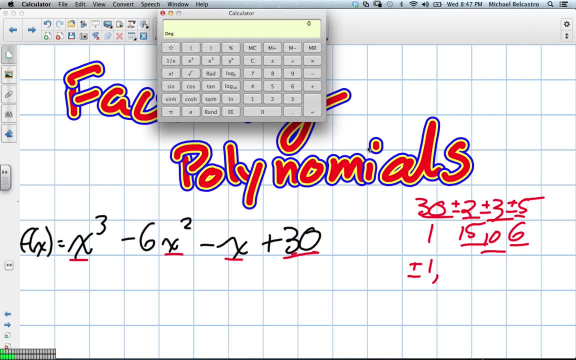 3 minus 7.. 3 squared is 8, added up, So that's negative 2, plus 8.. Negative 18, plus 30. That won't work. It's best when you get a calculator where you can write everything in at once. 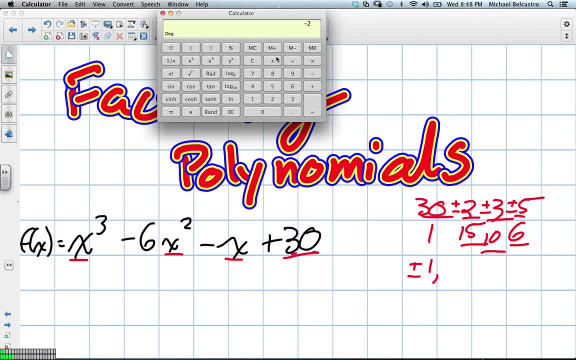 We could try: negative Negative 2 cubed is negative 8.. Negative 2 squared is still 4 times negative. 6 is 24, so we're minusing 24.. And then plus 2.. Ah, it's 30. Plus 30.. 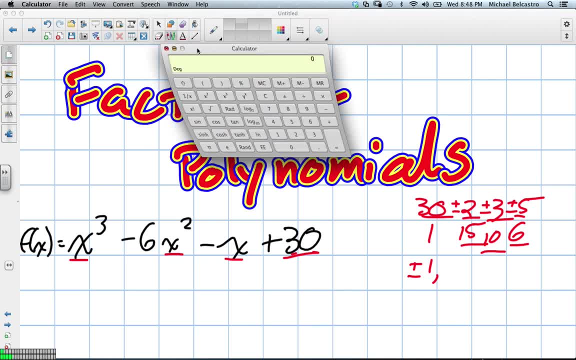 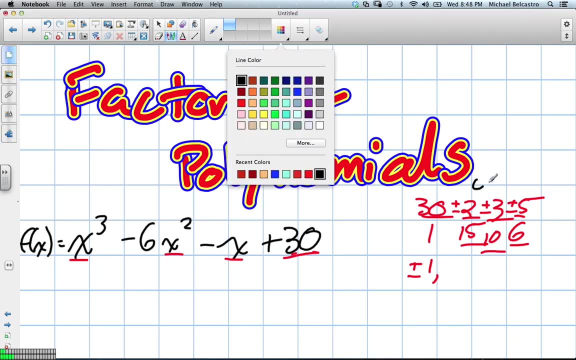 Perfect Equals 0.. So negative 2 is our…. see what I kind of did there. I know I did a lot of it in my head, but what we found was that negative 2 is a factor of this. okay, It creates a zero. So, because it's negative, 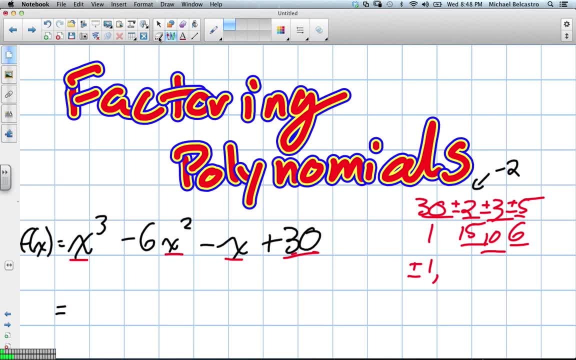 2,. what am I going to divide by? I'm going to be dividing by x plus 2.. This is going to be our factor. We're going to be dividing by this x plus 2, right, Because it's negative. 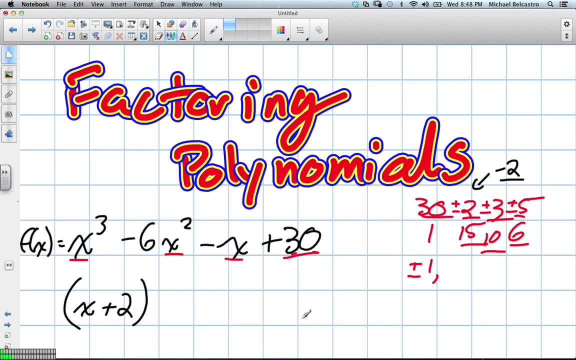 2.. And essentially what you could say is: it's our k value. So x plus k equals one of our factors and our factor is negative 2.. So to find out what- sorry, x minus k is negative, 2, okay, is equal to our factor. So, in order to get k, to figure out what k is going to, 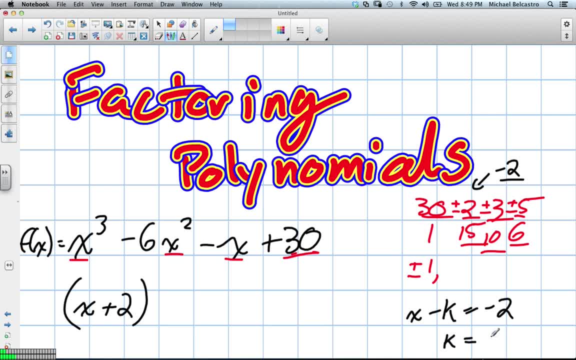 be, k is essentially going to be our positive 2.. So we take this long equation and we're going to divide it. We can use synthetic or long division. Which one do you want to use? Yeah, You find that easier. Okay, So in that case, 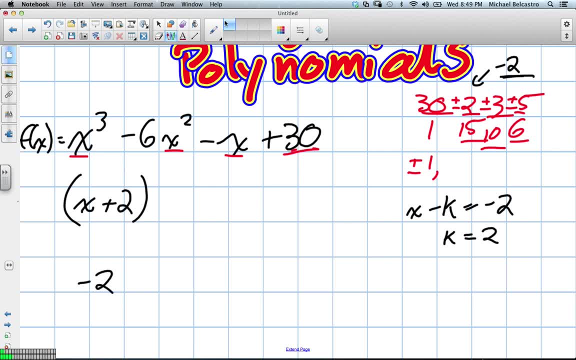 actually we keep our term k as negative 2.. We actually didn't have to try to change it back to x plus 2, but just realize we're essentially dividing by x plus 2.. We then write all the coefficients, the first one being 1,, next one being negative, 6,, next one being negative. 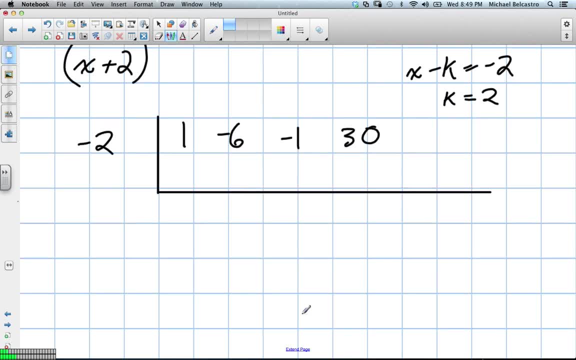 1, and next one being 30,. okay, We bring the 1 down and then we multiply it by negative 2.. So when we multiply by negative 2, what do we get? Negative 2.. Okay, and then we add: 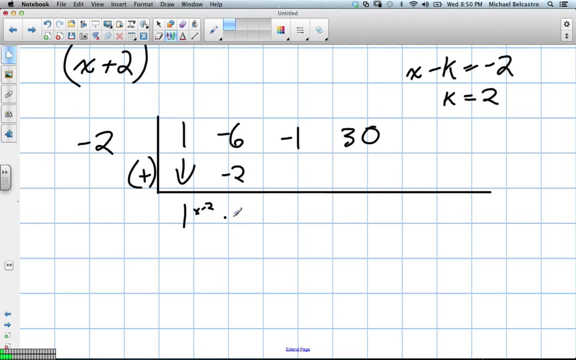 Negative 6 and negative 2?. Negative 8.. Okay, negative 8 times negative 2 gives us 16.. Yeah, positive 16.. Negative 1 plus 16 is 15. 15. Negative 2 times 15?. 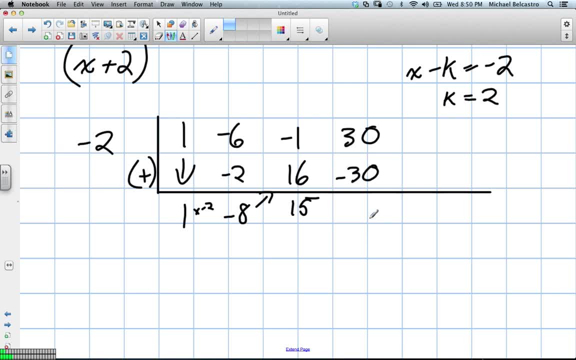 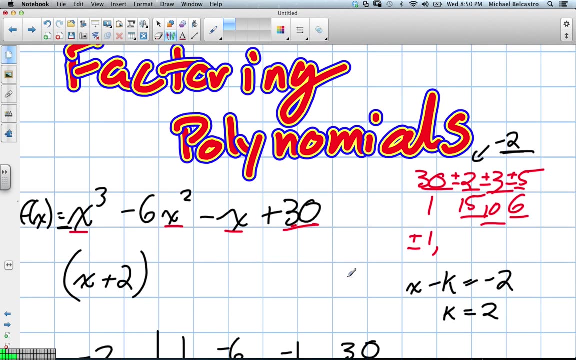 30.. 30. Sorry, negative 30. And what is our remainder? It should be because we took 2, and we discovered that it was going to be. it was going to create a 0. So there is no remainder here. So our equation: now we've actually taken a factor out of it, Our f at.